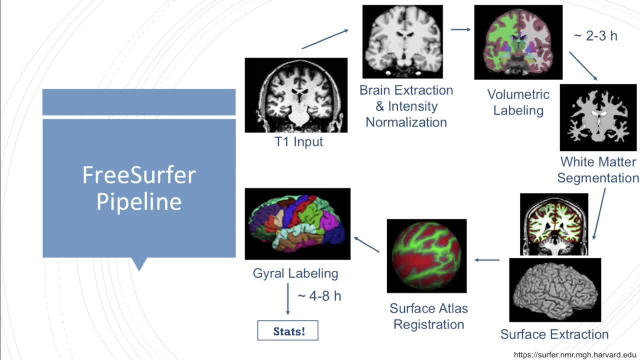 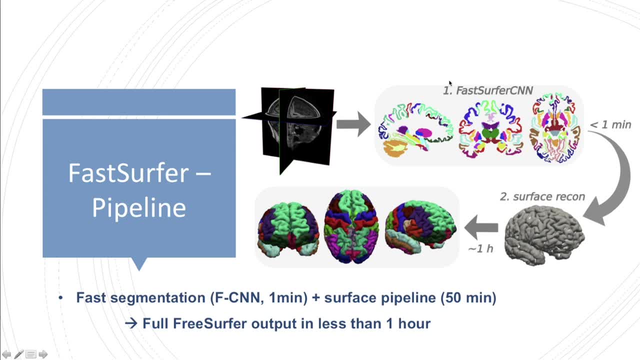 then get a full FreeSurfer output in a fraction of the time, And in order to do this, we use an advanced deep learning architecture called FastSurferCNN to create a whole brain segmentation into 95 classes in less than a minute, which basically mimics FreeSurfer's anatomical segmentation. 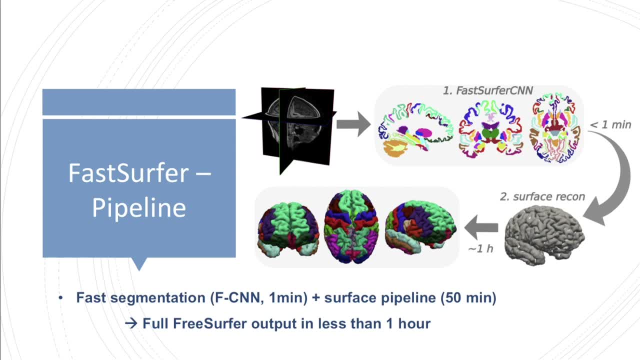 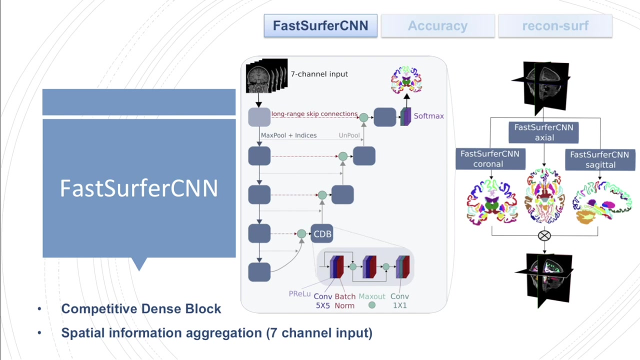 and cortical parcellation And then, building upon this high-quality segmentation, we generate a full FreeSurfer output, including cortical surface reconstruction, mapping of cortical labels and traditional pointwise and array thickness analysis, in approximately 60 minutes. FastSurferCNN is composed of three fully convolutional neural networks operating on coronal axial. 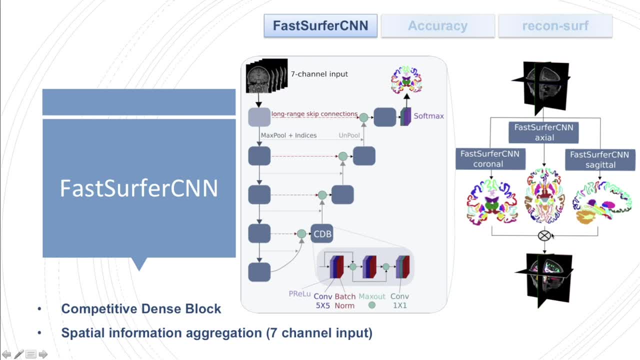 and sagittal 2D slice stacks. And a final view: aggregator. FastSurferCNN is a multi-layer network aggregation stage. Within each FCNN we incorporate local and global competition via competitive dense blocks that are depicted down here and competitive skip pathways. 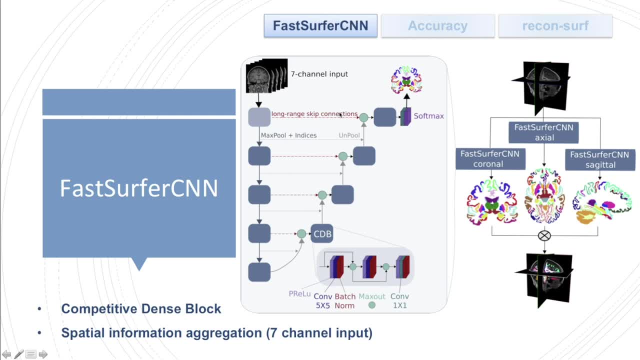 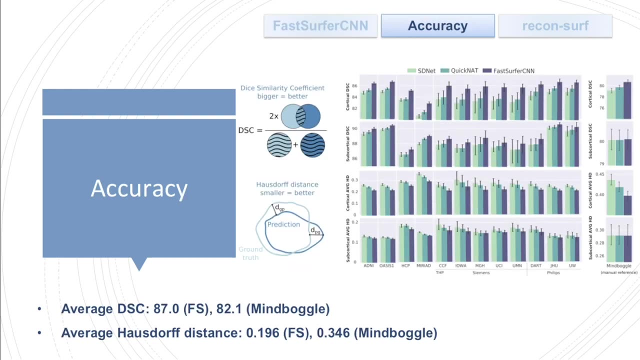 So we use maxout at the end of each long-range skip connection, As well as multi-slice information aggregation by using a seven-channel input, And these modifications specifically tailor network performance towards the accurate recognition of both cortical and subcortical structures, as can be seen in our accuracy analysis. 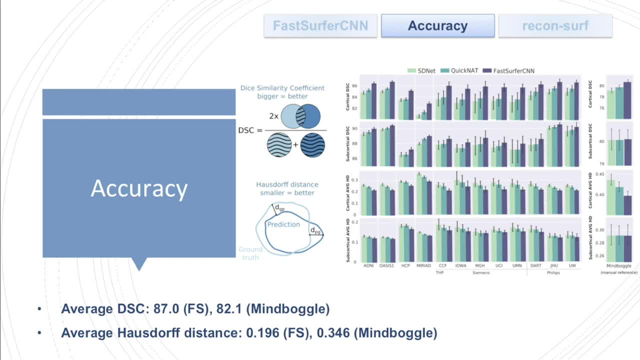 So here we compare the die score as well as the Hausdorff distance for the cortical and the subcortical structures. The cortical is always on top And compared to other deep learning architectures- FastSurferCNN, which is depicted in dark blue- 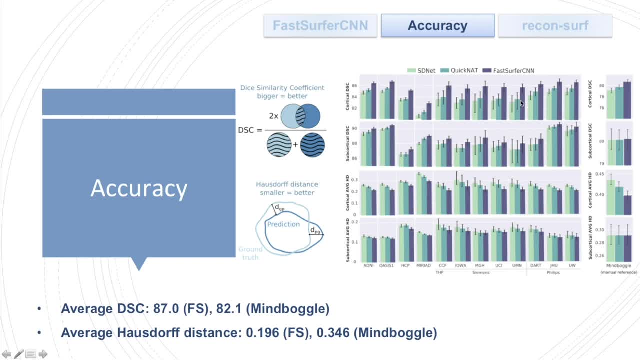 reaches a higher die score, Both for the cortical and the subcortical structures. The cortical is always on top And compared to other deep learning architectures. FastSurferCNN is a multi-layer network aggregation stage And here we compare the die score, as well as the subcortical as well as the subcortical. 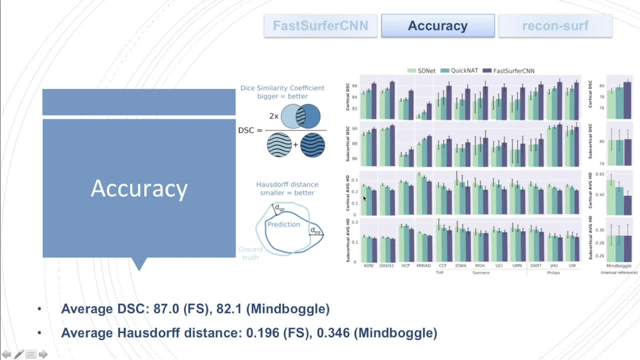 structures And a lower average Hausdorff distance again for both the cortical as well as the subcortical structures. And this is also with respect to FreeSurfer as a reference, which is depicted here on the left for multiple data sets, as well as a manual standard here on the right. 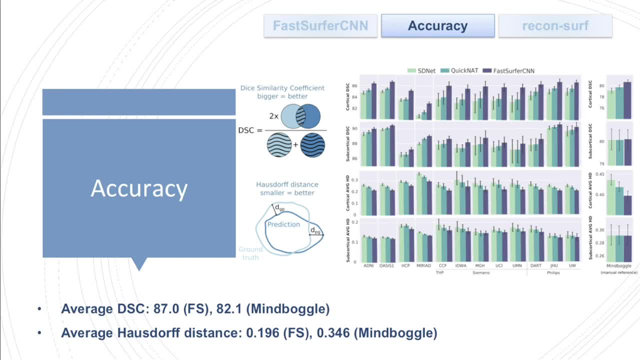 On average. FastSurferCNN reaches a die score reaches a dice of 87 for FreeSurfer and 82.1 with respect to MindBoggle. as a reference, The average house of distance is 0.196 with respect to FreeSurfer and 0.346 with respect. 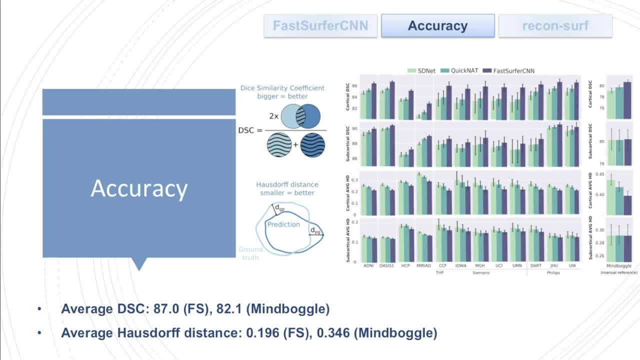 to MindBoggle. So overall we see that FastSurferCNN outperforms other deep learning architectures by a significant margin, both with respect to FreeSurfer as a reference and the manual standard, and also that it generalizes quite well across a number of different data sets. 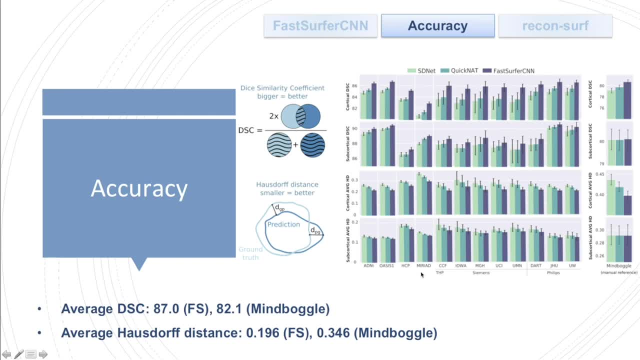 which include different disease states, different age groups as well as different scanner types. already, One additional advantage of using FastSurferCNN compared to a standard FreeSurfer run is that, because segmentation is generated just based on the MRI volume input, many steps. 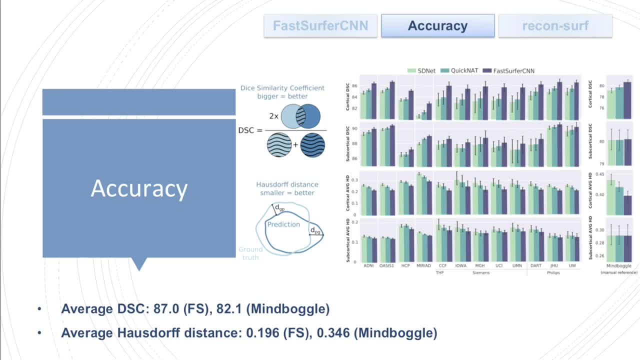 that are used in the traditional FreeSurfer can be performed within the same data set. This is important because the data set that we are currently using is not necessarily the same as the data set that we are currently using. For example, if we look at the single-spectral embedding, we can see that the two non-constant 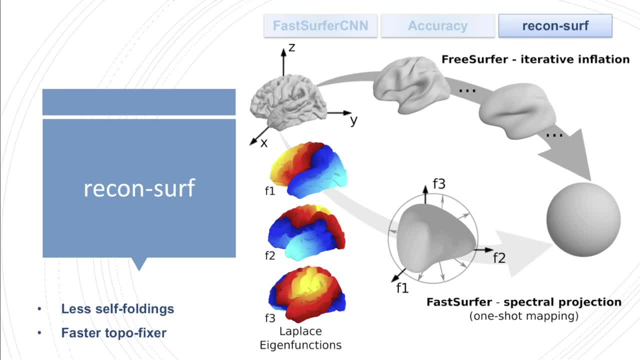 eigenfunctions of the first and third. non-constant eigenfunctions have all become obsolete, such as skull-tripping and non-linear atlas registration, which already results in a speed up of the entire pipeline. In addition, within Rec&Serve we introduce an alternative to FreeSurfer's 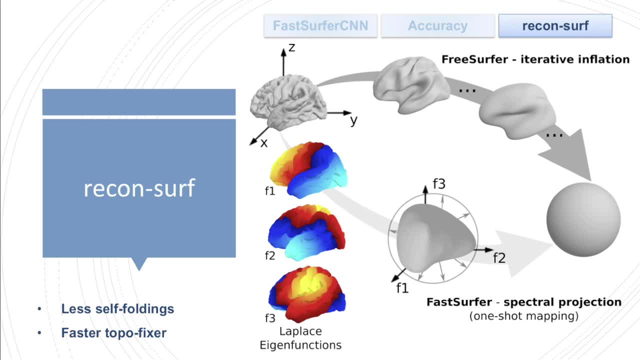 traditional iterative spherical inflation process, which is depicted here at the top. We use the Laplace-Beltrami operator to parameterize the surface smoothly. Then we quickly generate the final spherical map by scaling the 3D spectral embedding vector to unit length, which then results in our sphere. This process in turn reduces cell. 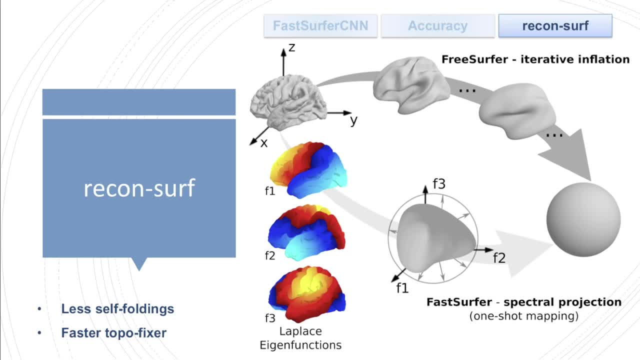 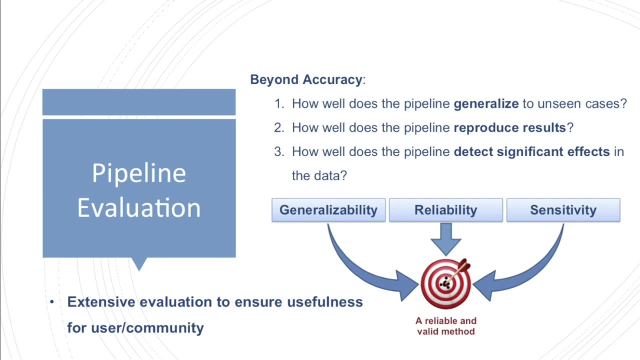 foldings and results in a slightly faster topology. In order to ensure that FastSurfer is, as a whole, not only accurate but also sensitive and reliable method, and to ensure its usefulness to the neuroimaging community, we extensively validated our pipeline with respect to three main aspects, and that is: 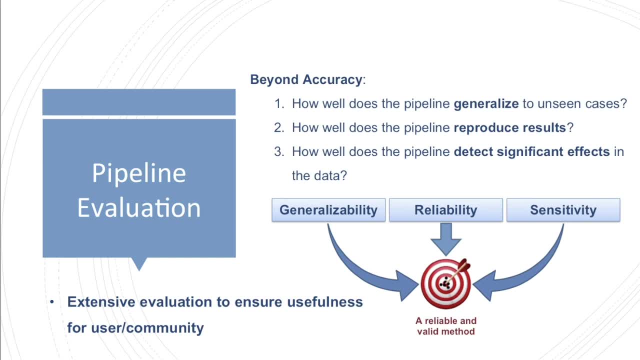 one: how well does the pipeline generalize to unseen cases, for example, different data sets, age ranges, disease states, vendors and so on? Two: how well does the pipeline generalize to unseen cases, for example, different data sets, age ranges, disease states, vendors and so on? 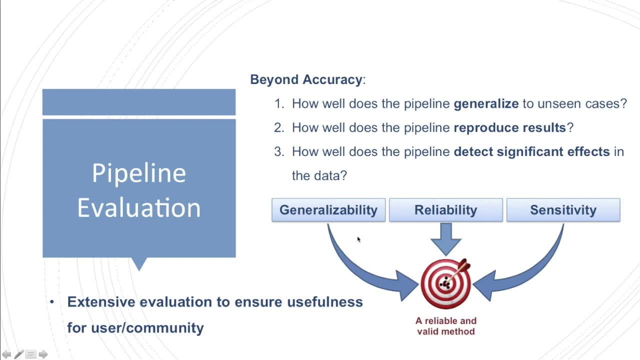 Which relates to the topic of generalizability. Second, how well does the pipeline reproduce results between scans with minimal anatomical variations- For example, it's the same subject is scanned twice within a short time frame- which relates to a reliability of the method. And third, how well does the pipeline detect? 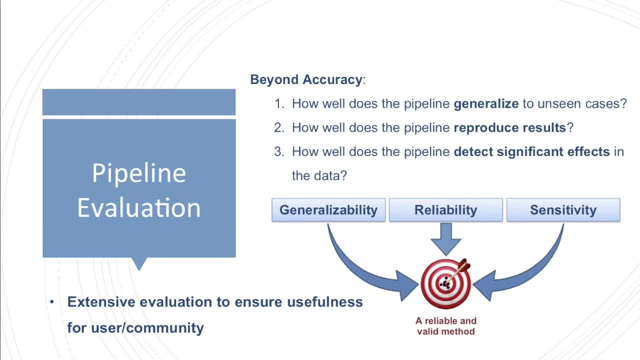 significant effects in the data, for example, changes or differences associated with disease states or aging effects, effects which relates to the sensitivity of the method. We will now inspect these three aspects to judge FastSurfer's performance in comparison to FreeSurfer. 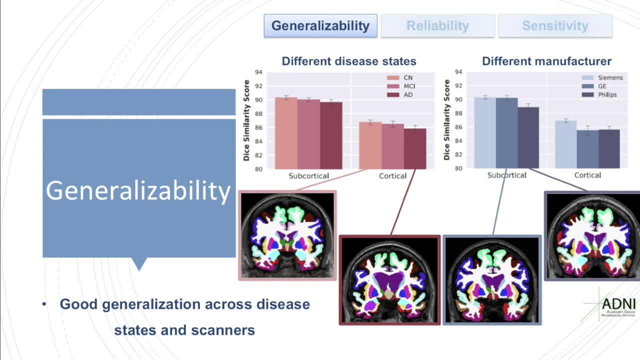 So first off, we used subjects from APNI to determine how well FastSurfer generalizes to unseen cases of different disease states shown here on the left. so this is my similarity score- and manufacturers here on the right- with respect to FreeSurfer. 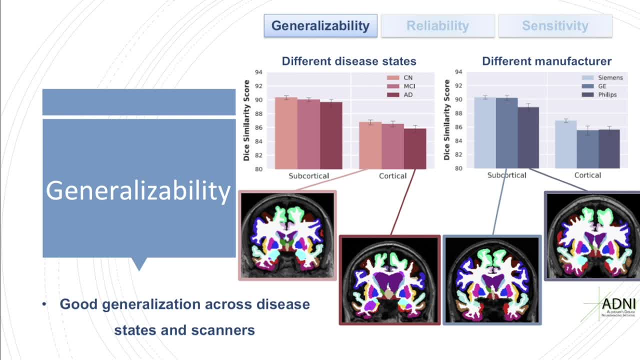 The segmentations of both methods, FastSurfer and FreeSurfer- closely resemble each other, as can be seen by the high dial score for the subcortical as well as the cortical structures. The segmentations deviate a bit more for extreme cases, like the Alzheimer patients, which 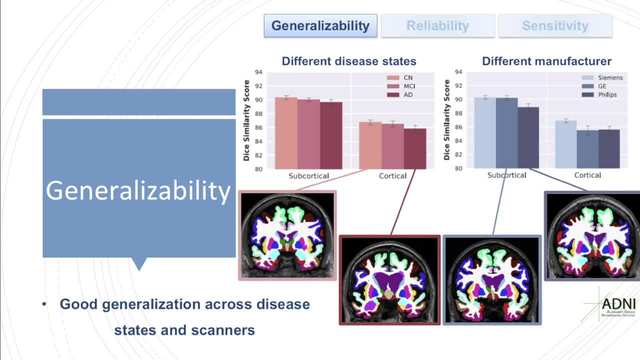 is not necessarily a quality deficit, but might actually be due to noisy data, increased motions in these patients or also blurring of the white-gray metaborder. In this example, we can see that the segmentations of both methods- FastSurfer and FreeSurfer. 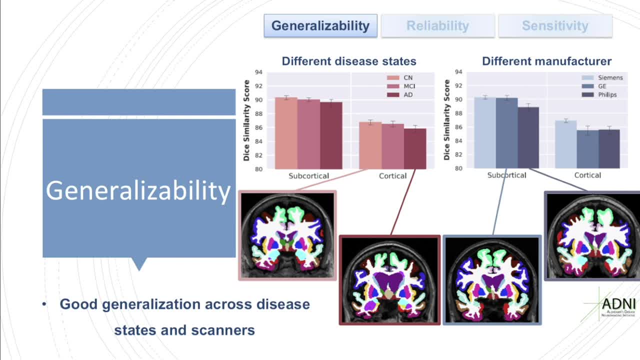 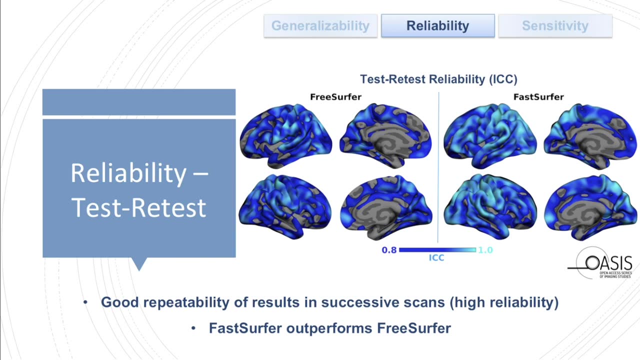 are relatively similar and overall we can still say that both methods stay relatively similar to one another and we have a good generalization across disease states and scanners for FastSurfer. In the second analysis we use the OASIS-1-Test-Retest component to calculate the intraclass correlation. 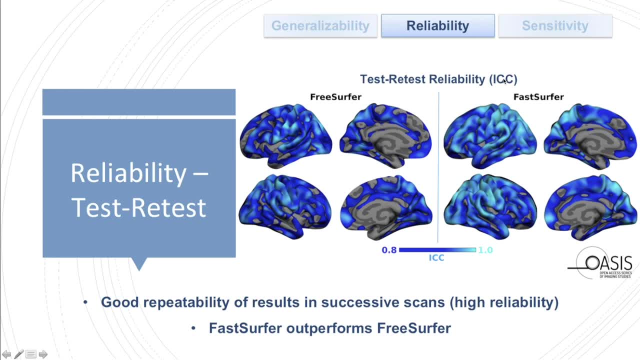 coefficient. so the ICC, which is an estimate of the agreement between results of scans with minimal anatomical variation. Here are the results for FreeSurfer, On the left and on the right. we have FastSurfer and you can see that for FastSurfer we get. 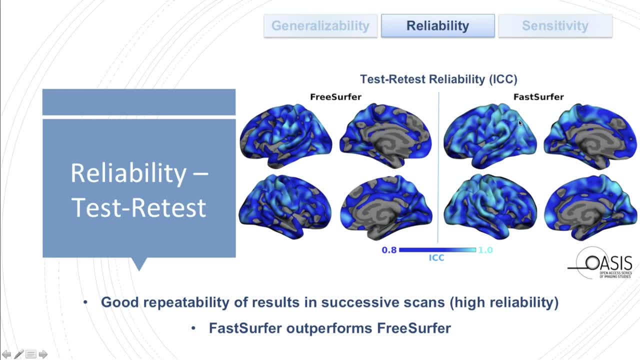 larger areas with higher ICC, so light blue values compared to FreeSurfer, and in addition we see that FastSurfer is highly reliable with a close agreement between the cortical sickness measurements across the entire cortex. so there is basically no area that is not. 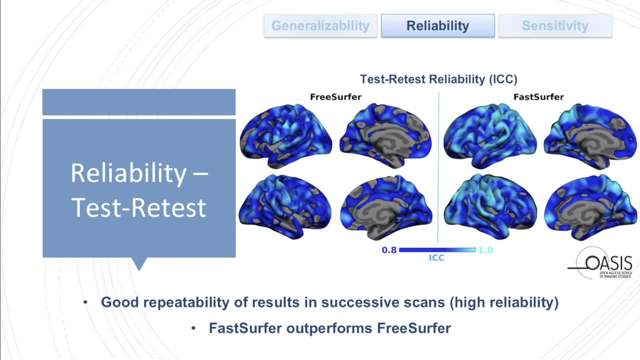 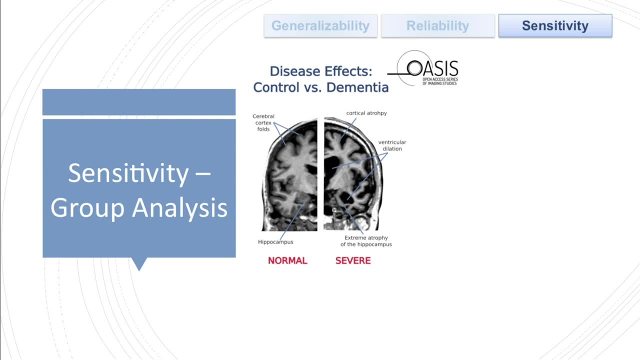 blue in this case. So the entire cortex is an ICC of above 0.8.. Finally, we use the cross-sectional part of OASIS to determine how well FastSurfer is capable of reproducing known disease effects in a group study between control and dementia. 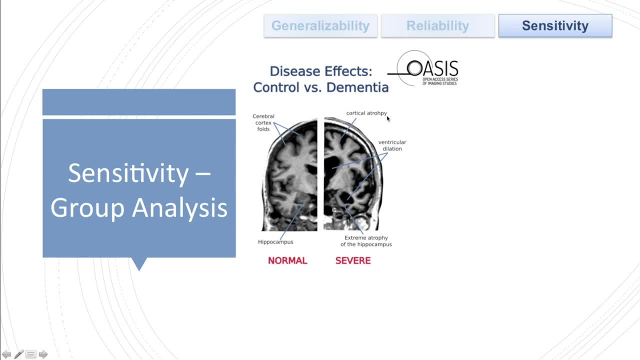 patients, such as, for example, cortical atrophy, ventricular dilation or atrophy of certain subcortical structures, like, for example, the hippocampus, And with FastSurfer we are actually indeed able to find reduced cortical thickness in. 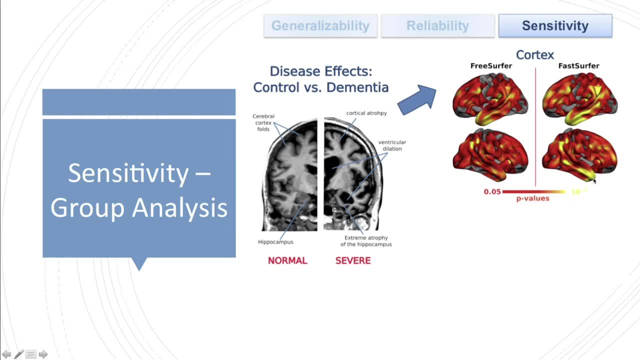 regions associated with dementia, as can be seen here, indicated by the p-value with high sensitivity, for example in the temporal lobe, and that also we have increased sensitivity relative to FreeSurfer. again, The same is true for the subcortical volume differences in this case, 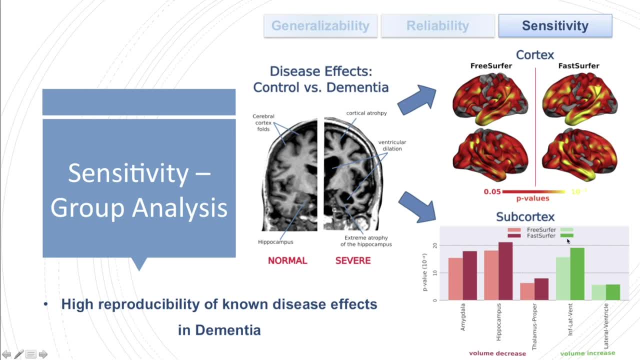 Here FastSurfer is darker. Okay, So we can see that FastSurfer has a lower p-value, which is indicated here by a larger bar for differences between the amygdala, hippocampus and thalamus, which are basically 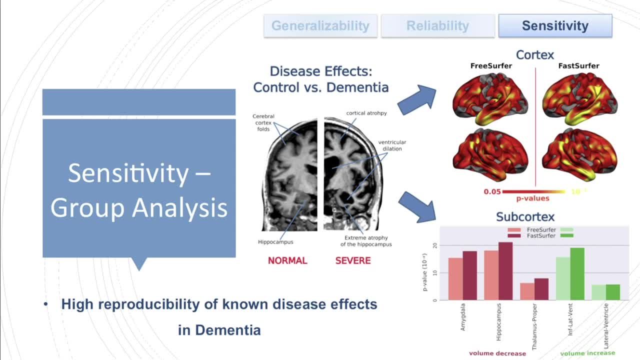 decreased in dementia patients compared to controls, as well as ventricles, which are enlarged, And again we see that FastSurfer has an increased sensitivity compared to FreeSurfer. So in total, we are able to robustly reproduce known disease effects. 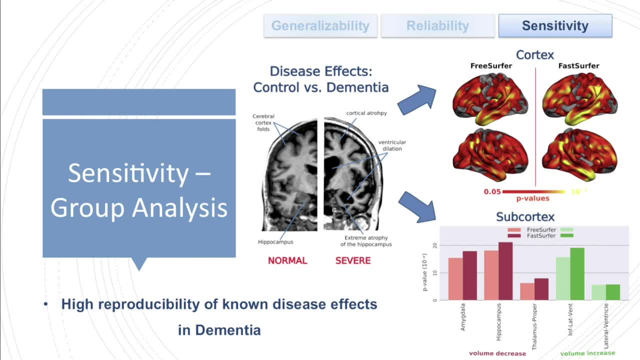 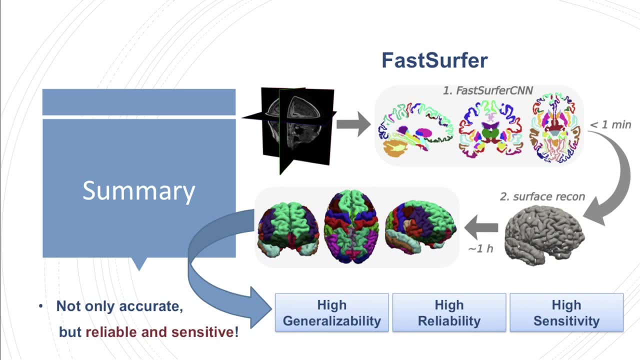 So overall, we could show that FastSurfer is indeed not only an accurate tool but also reliable, sensitive and generalizes well to unseen cases and is, as such, hopefully of use to many of you. That was my talk. Thank you for your attention. 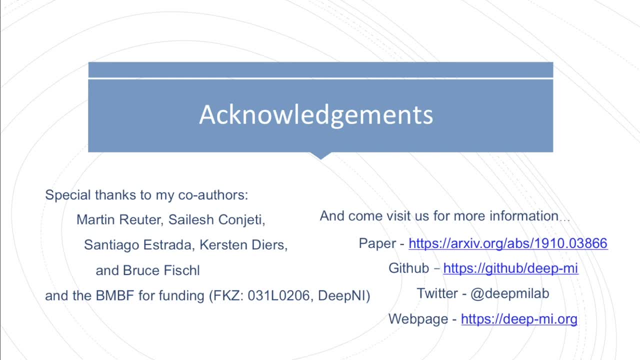 And, of course, I would like to thank all the people who made this work possible, especially my fellow co-authors Martin Reuter, Salish Kanjeti and Santiago Ramos. Thank you, Bye. Good day, Andajo Estrada, Kerstin and Bruce, as well as the BNBF, for our